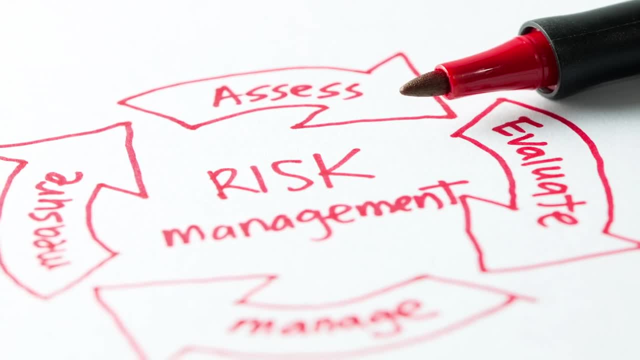 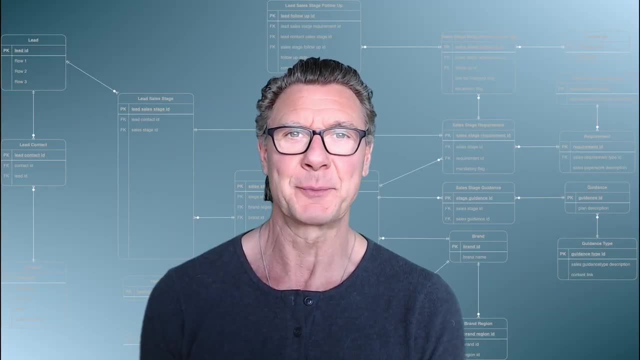 workflows, arrows, et cetera, to depict things in business, how we do things, the steps and the sequences of achieving something In life. we often describe ourselves as a process. If we asked at the party to describe a process, we would say that it's a process. If we asked at the party to 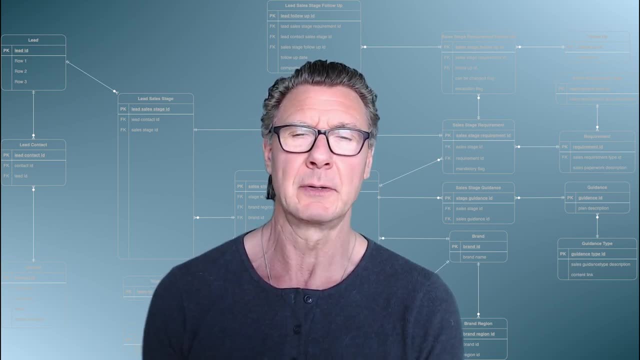 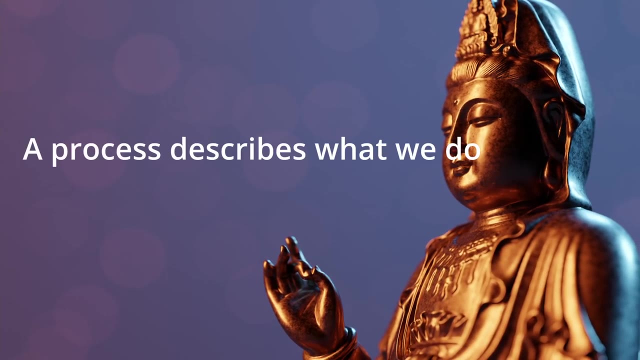 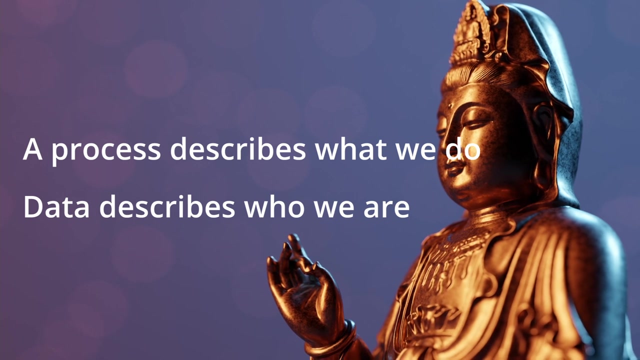 describe ourselves. we often describe what we do, not who we are. Now it's getting philosophical. A process describes what we do. Data describes who we are. Data can exist without the process, whereas a process must have data to exist. You could say that data is persistent. 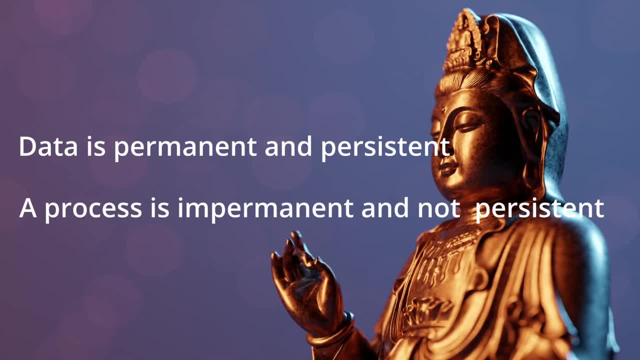 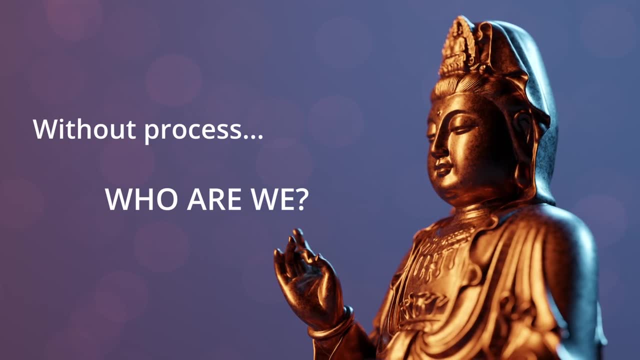 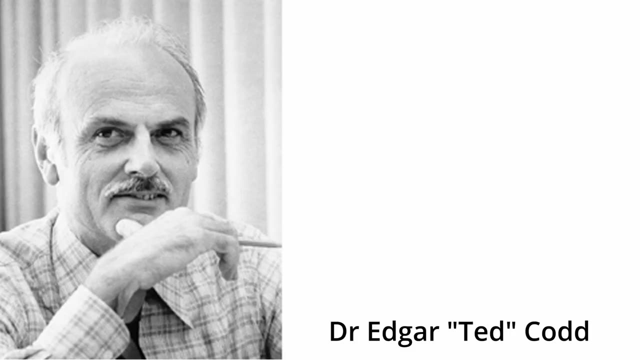 whereas a process is not. That raises the question. so, without the process, who are we? Very philosophical and certainly worthy of a serious dinner conversation. But Edgar Codd entered the scene and he wanted more than great dinner conversations. He reduced data and data relationships into mathematics and in 1970 he released the 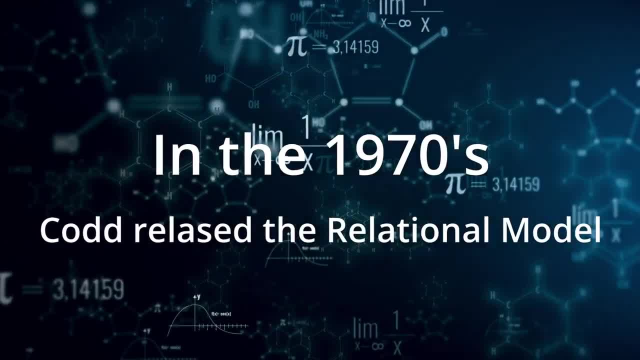 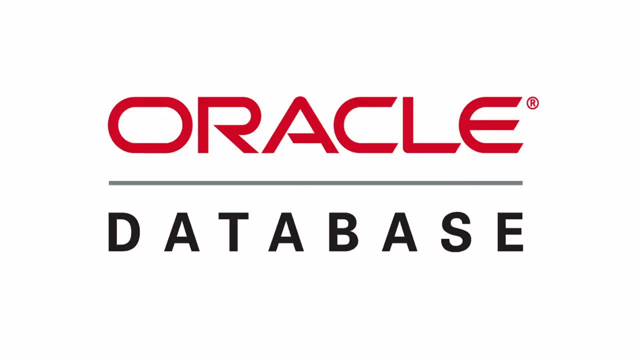 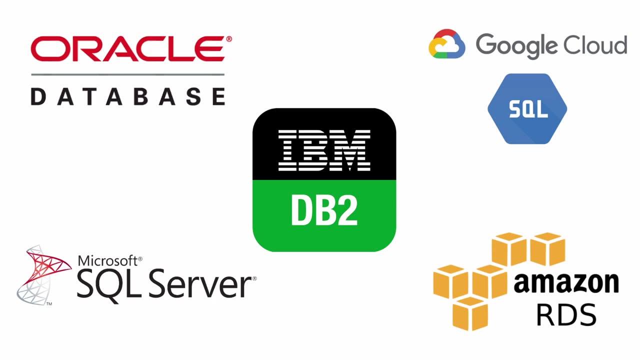 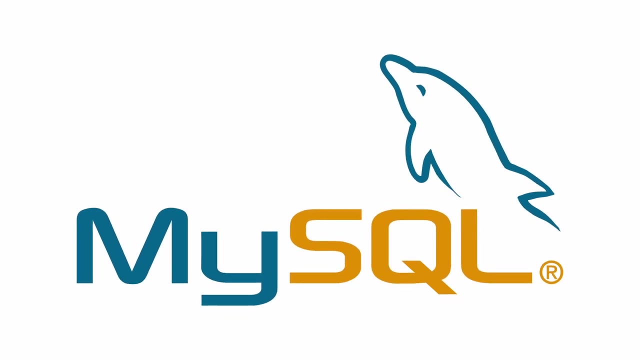 relational model, which is a systematic approach of connecting and maintaining data based on mathematical rules. Technology companies like Oracle, IBM, Microsoft, Amazon, Google used his relational model to create their own relational databases. Popular open source databases like MySQL are also based on it. 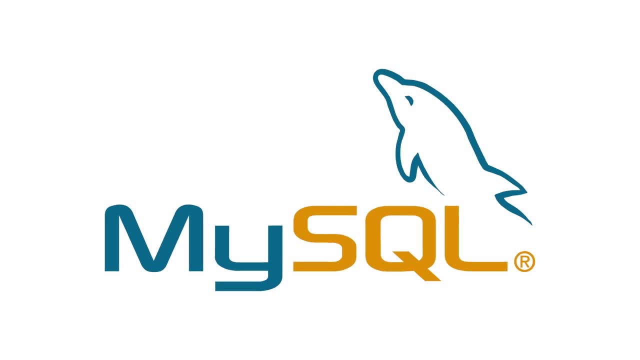 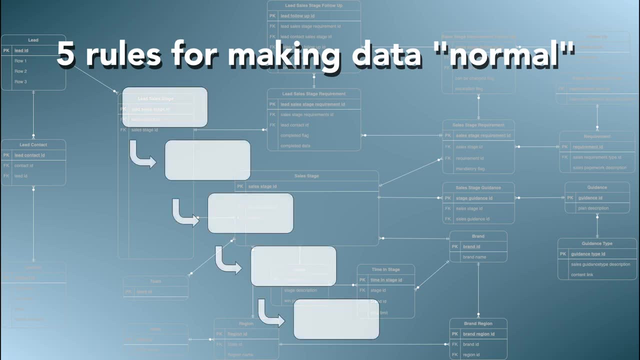 But that's all technology. Let's forget about the technology for now. Dr Codd provides five rules to normalize data, where each rule builds on the other, starting with first normal form and ending with fifth normal form. Normalization is a gateway into deeper data understanding because it addresses the things 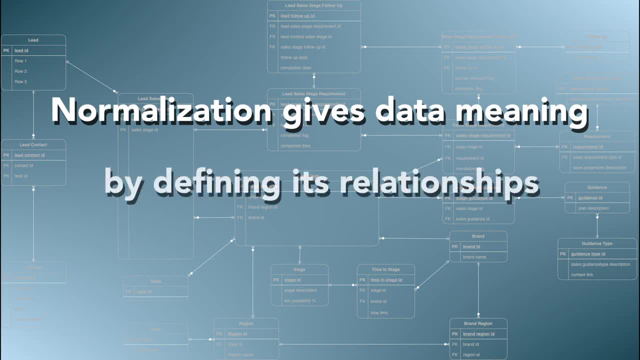 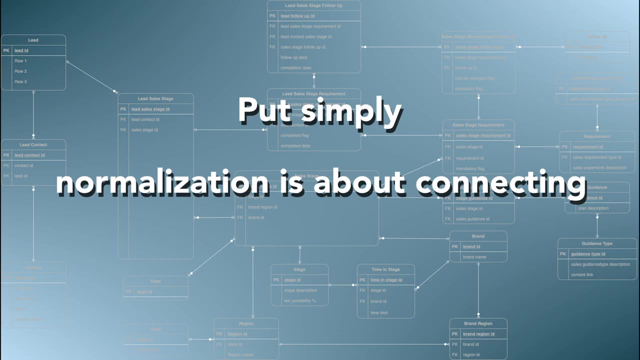 that give data most meaning, which is its relationships with other data. The magic of data lies in its relationships and types of relationships, called cardinality. Put simply, normalization is about connecting data to other data. Normalization is about connecting data in the right way. 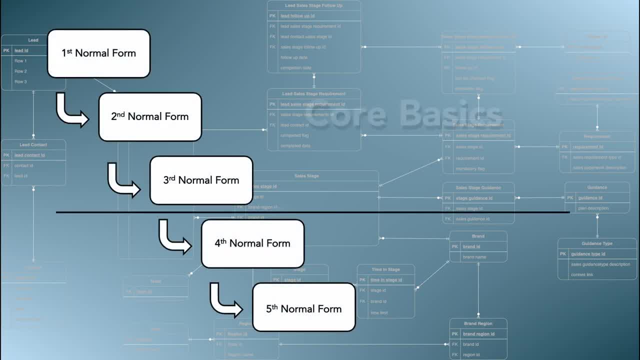 The first three rules of normalization are about core basics, whereas the latter two deal with exceptions. Hence, for practical reasons, normalization typically refers to third normal form, And remember to be in third normal form. it must also be in first and second normal form. 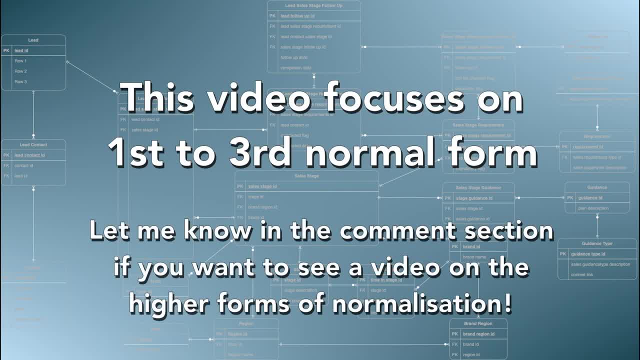 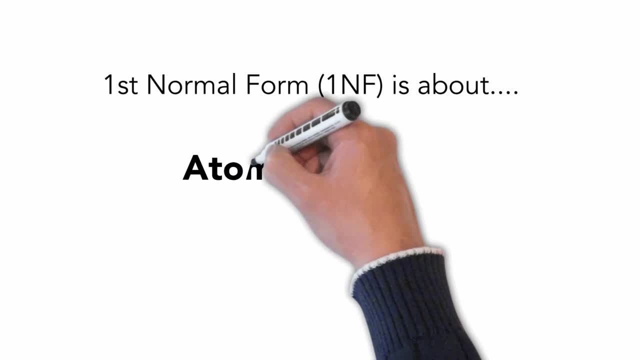 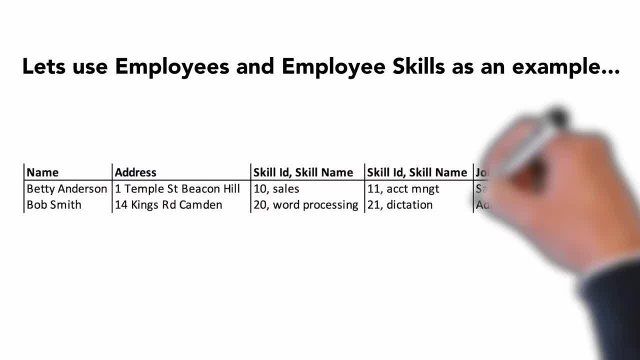 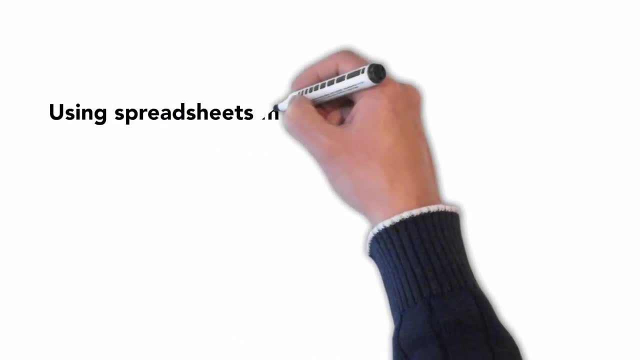 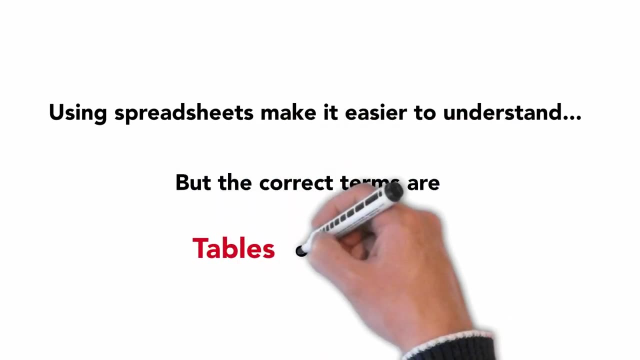 Let's say we want to model employees and their skills and we have been handed this spreadsheet of data with the task of normalizing it. I've used spreadsheets as an example to make it easier to understand, but the correct term is either to use table or entity. 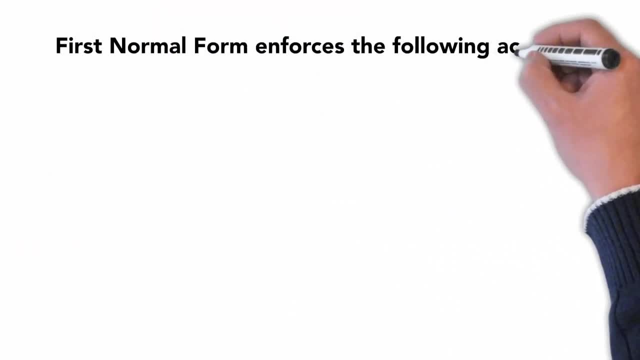 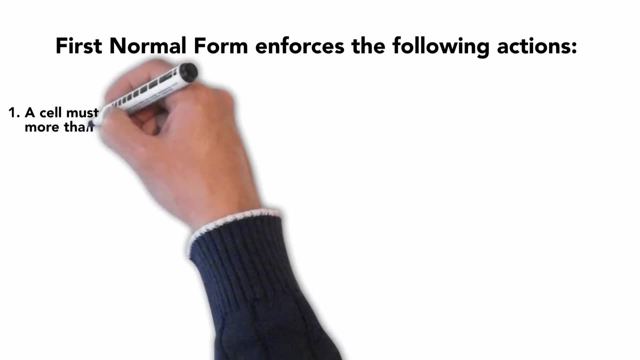 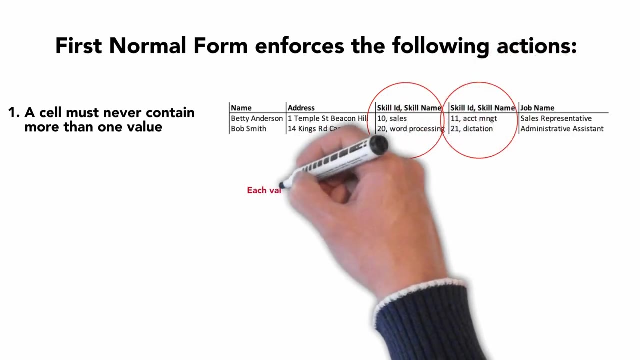 But the correct term is either to use table or entity First. normal form specifies that the following actions need to be taken on the data Number one: Each cell may never contain more than one value. For example, a cell cannot contain both skill id and skill name. 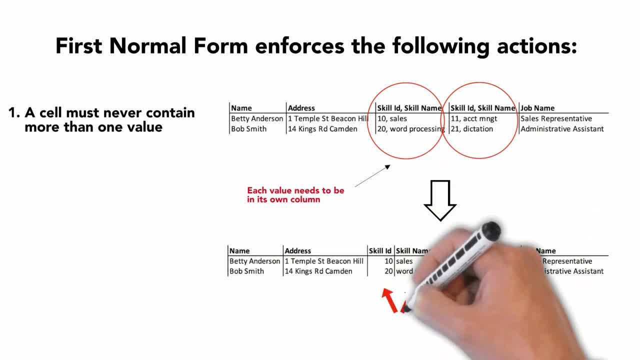 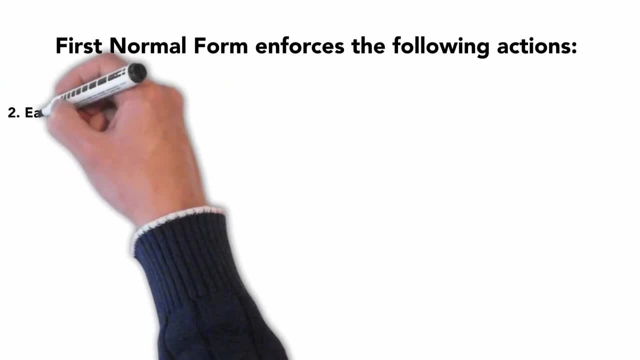 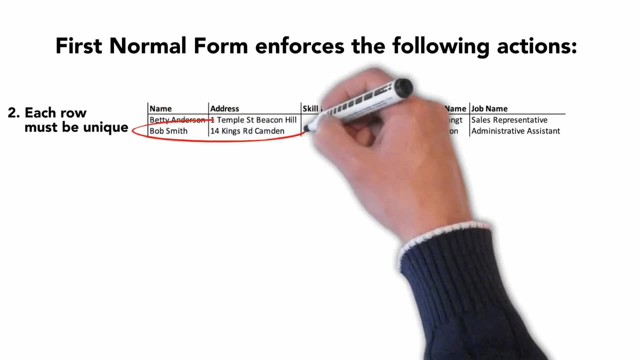 As a result, we need to split into separate columns. 2. Key upgrades at prime form, Second form, First normal form specifies that the following actions need to be taken on the data Number 2. Each row must be unique, That is, one column or a combination of columns must be able to uniquely identify the row. 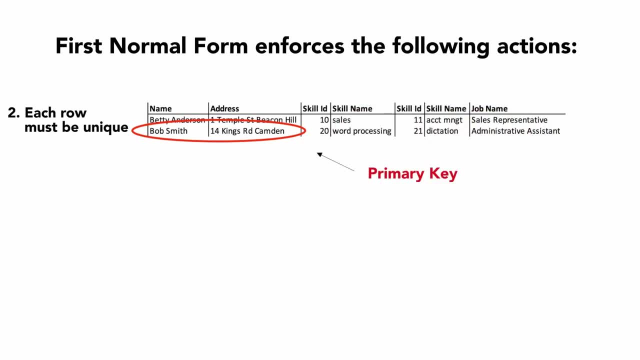 This is called the primary key. In this example, name and address would be a potential primary key, Yet often the primary key is system generated. In our case, we will add a computer generated primary key. The primary key is of great importance and features prominently in all other normalization rules. 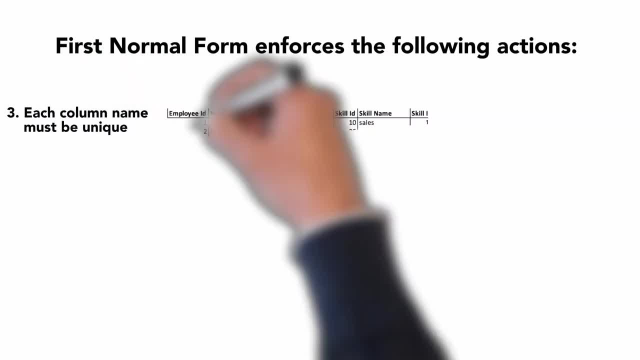 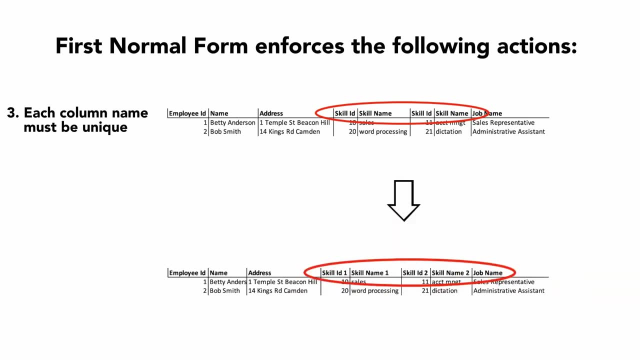 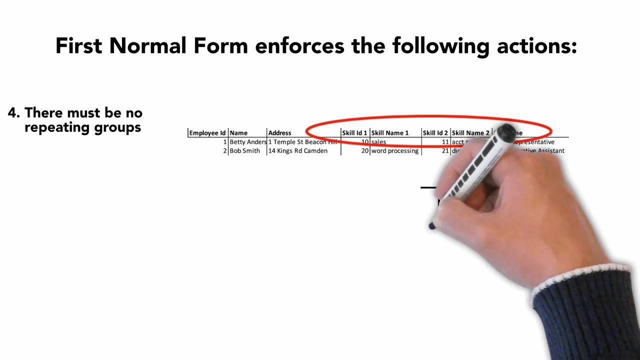 3. It also means that each column name must be unique, And in this case we need to rename our skill columns to make them unique. And 4. There must be no repeating groups. Repeating groups are removed and put into a new spreadsheet or table. 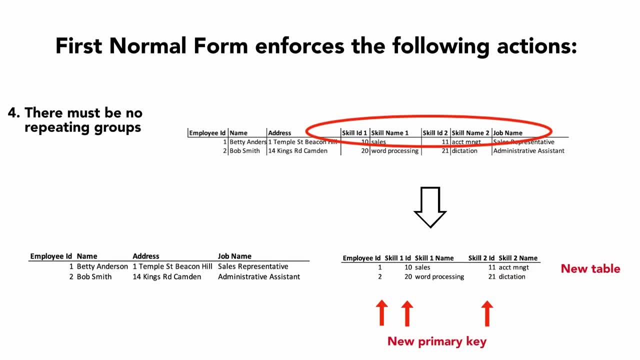 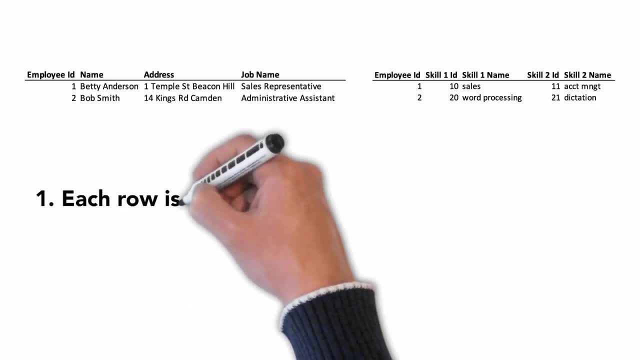 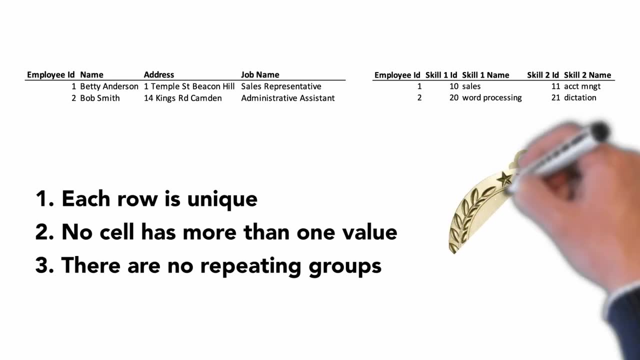 Now we have two spreadsheets, or tables, with nice rows of data. Each is uniquely identified, Each has no more than one value in each cell And there are no repeating groups. Yay, Welcome to first normal form. but the fun doesn't stop here. 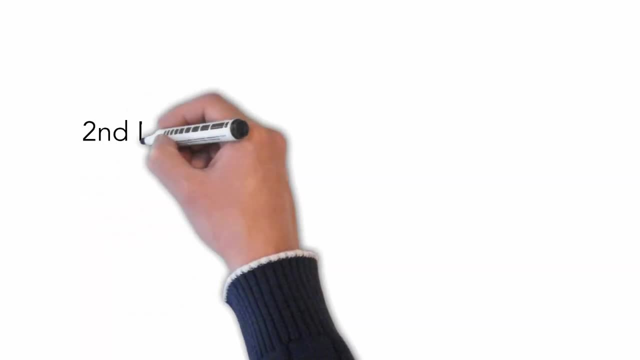 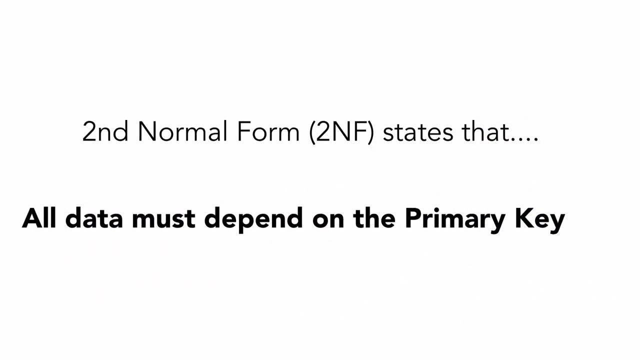 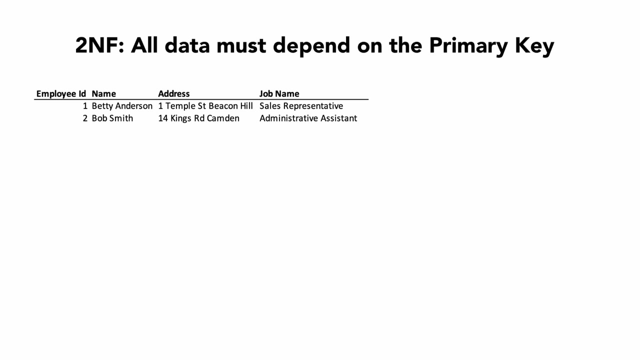 2. Second normal form enforces new rules and states that All tables must be unique. Data must depend on the primary key. So let's first examine spreadsheet 1. Name and address and job names are all related to employee ID, So it's already in second normal form. 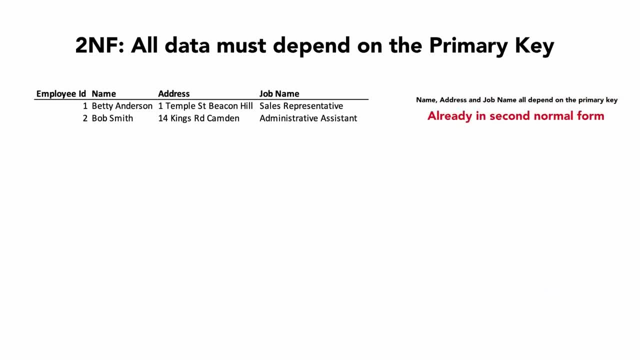 Yay, That's great, But what about the second spreadsheet? Skill name relates to skill ID but not to employee ID. 2. Second normal form stipulates that Any column that don't depend on the whole primary key must be split into its own spreadsheet or table. 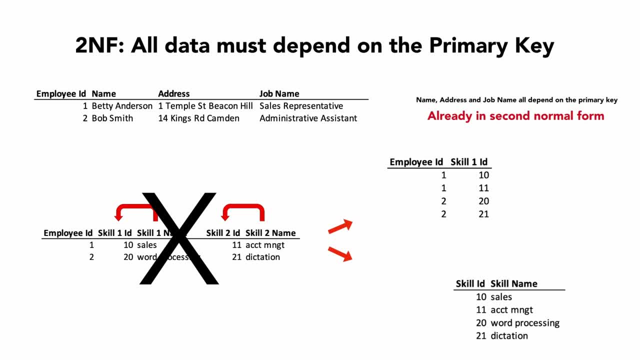 So we need to create one more, called employee skill, A primary key that links to other spreadsheets or tables are also called a foreign key. So in this case, employee ID is the foreign key of employee And skill ID is the foreign key of skill. 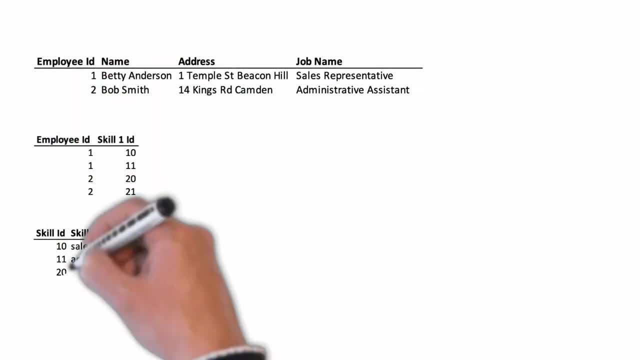 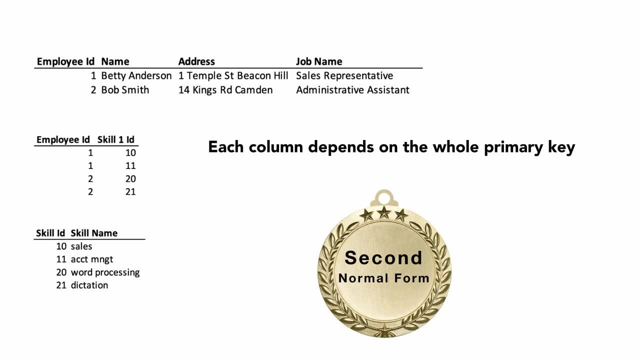 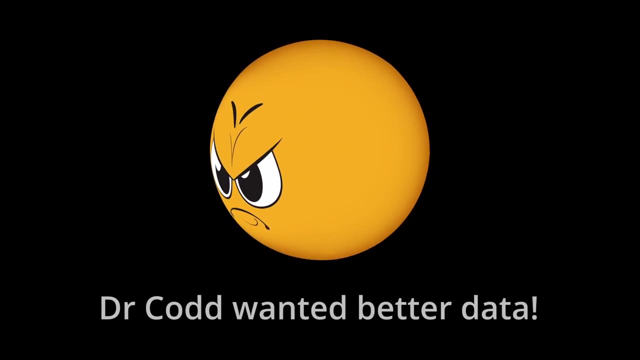 Now I have three spreadsheets or tables with nice rows of data where each column depends on the whole primary key. Yay Again. welcome to second normal form. But Dr Codd still wasn't happy and introduced a set of tighter rules called third normal form. 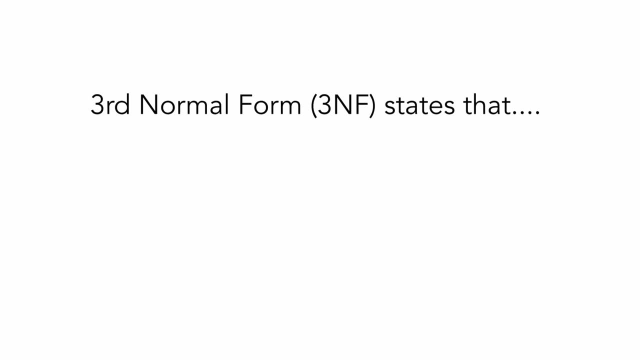 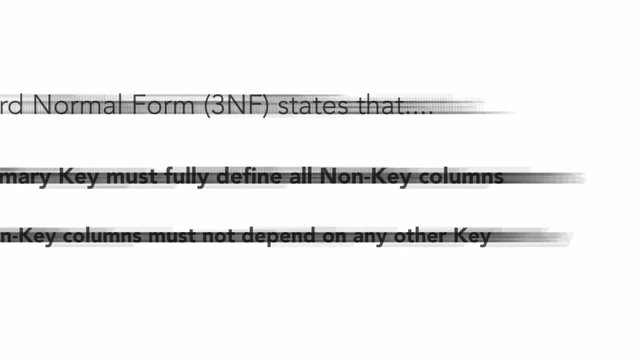 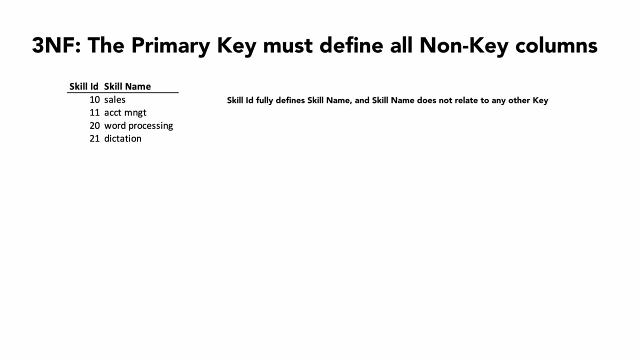 Third, normal form also focuses on the primary key and states that The primary key must fully define all columns and columns must not depend on any other key. So let's examine our spreadsheets again. In skills, skill ID defines skill name and skill name does not relate to any other key. 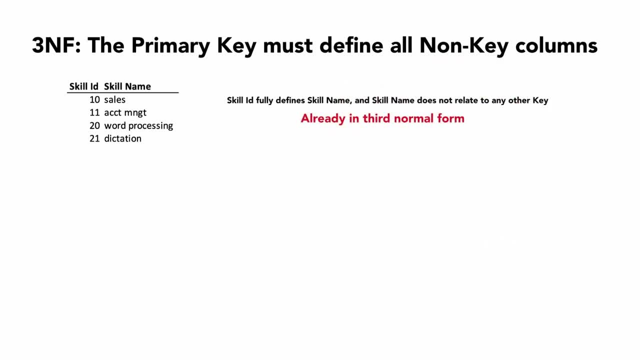 So it's satisfied third normal form In employee skills employee ID and skill ID has no other columns and hence satisfied third normal form In employee employee ID defines name and address and name and address do not relate to any other key and hence satisfied third normal form. 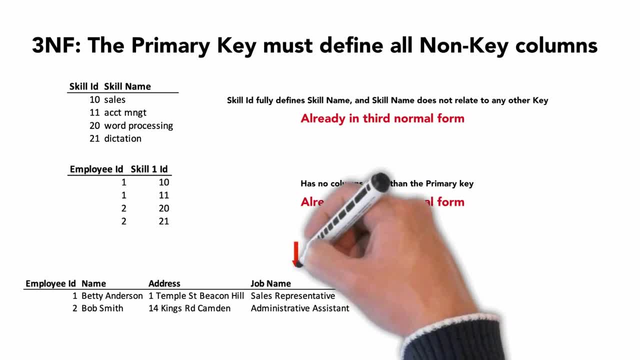 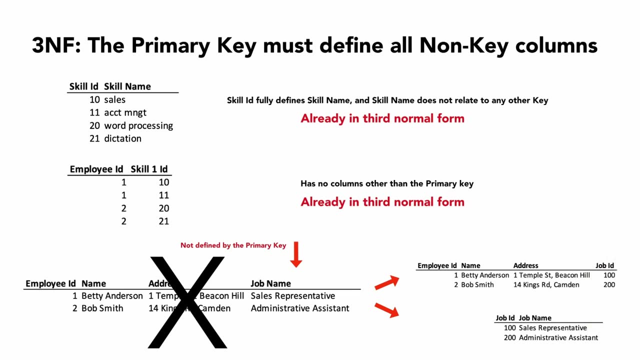 But employee ID does not define job name, hence violating third normal form. This means that job name needs to be split into its own spreadsheet and table And, for consistency, we have created a computer generated job ID. Because the job ID links employee and job, we need to create a new column, job ID, in employee. 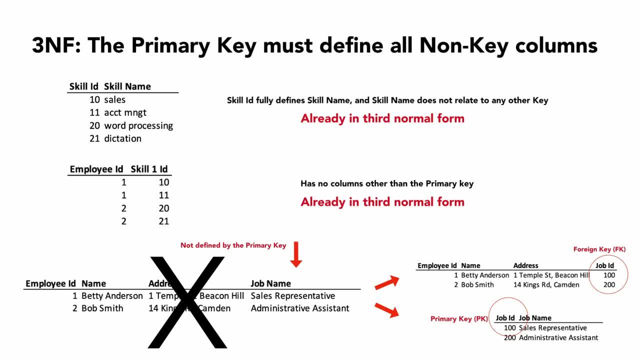 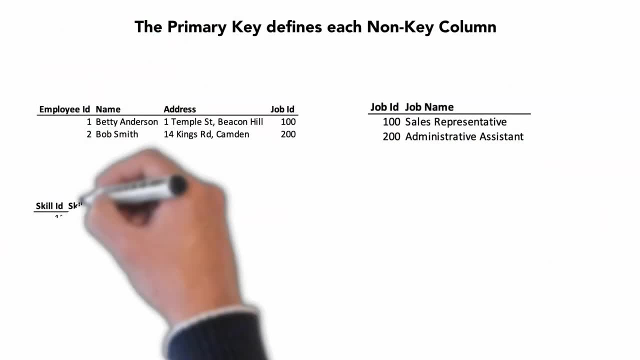 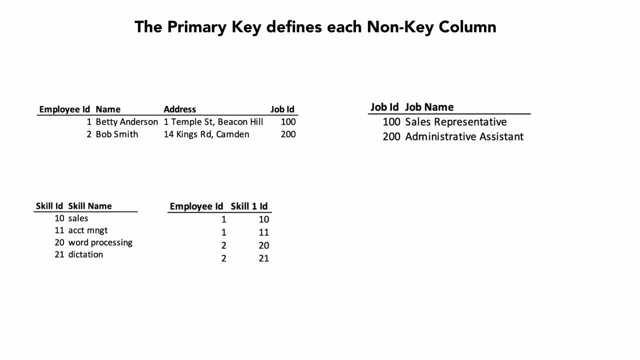 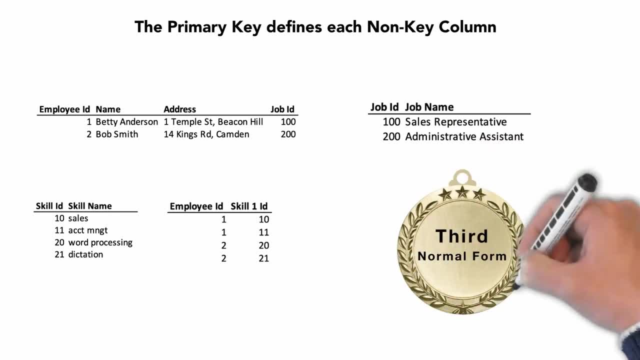 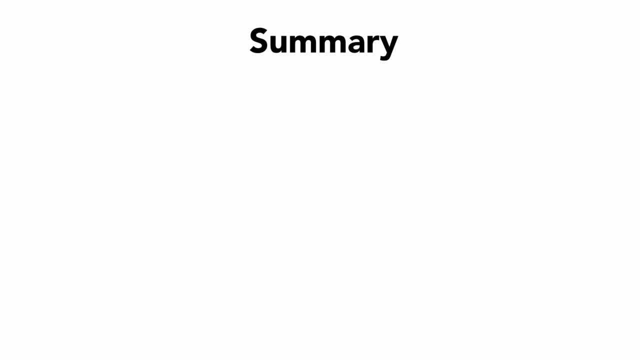 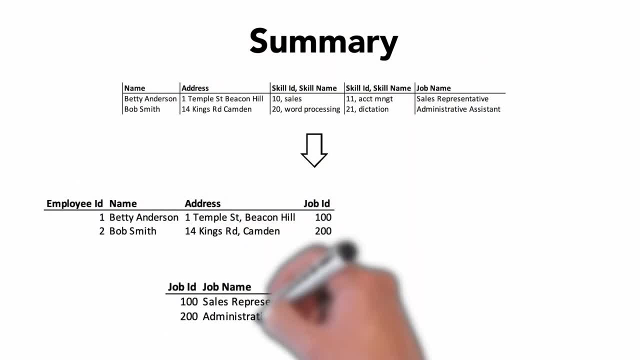 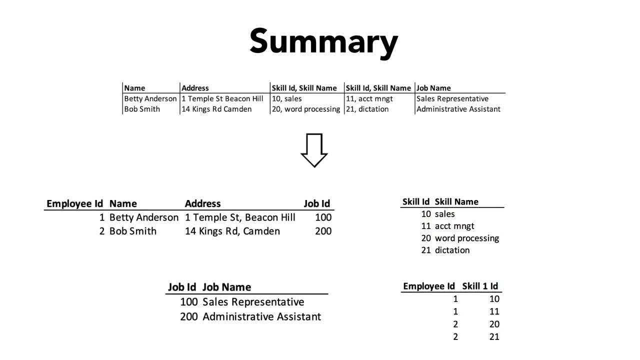 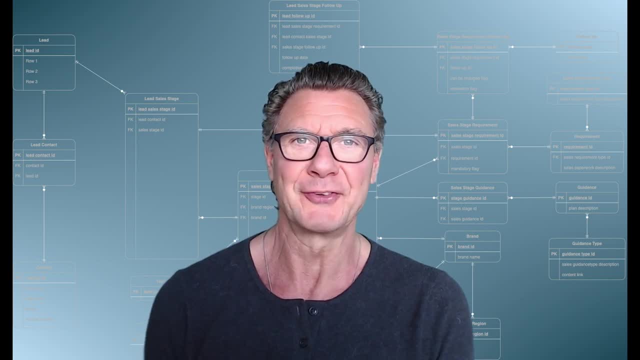 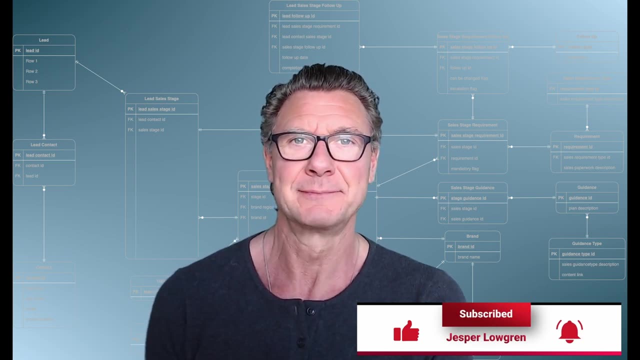 Now we have four spreadsheets or tables with nice rows of data. Now we have four spreadsheets or tables with nice rows of data and how to normalize data to third normal form. and if you enjoyed this video, please hit like and subscribe. hope to see you in my next video.